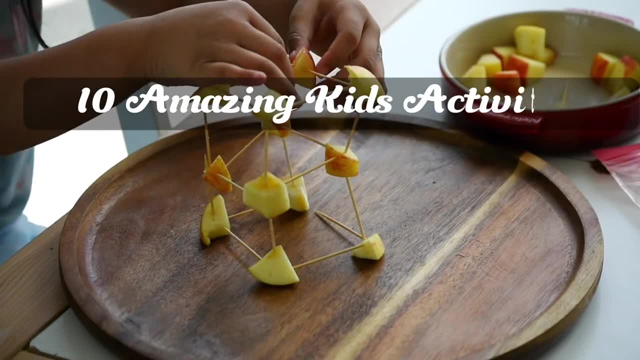 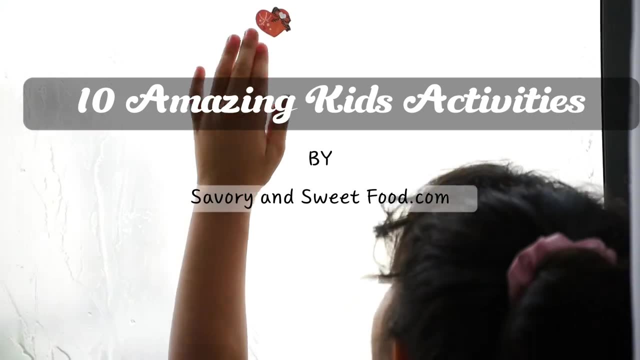 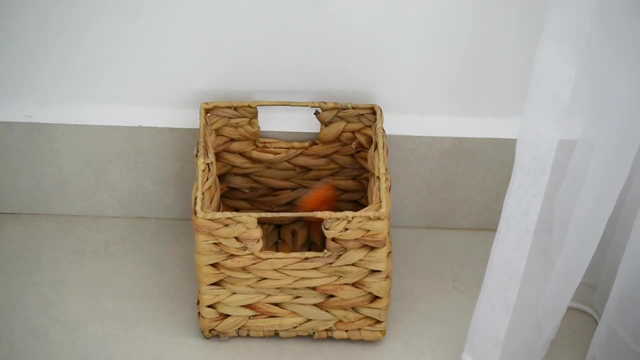 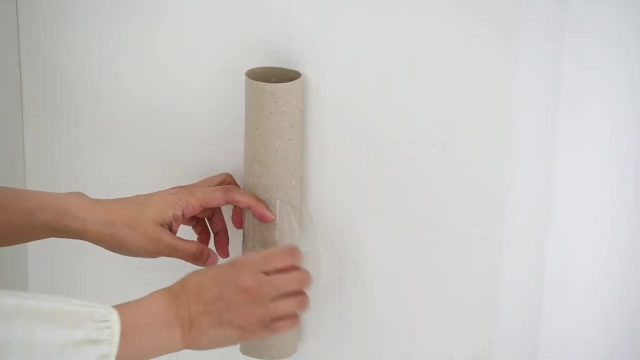 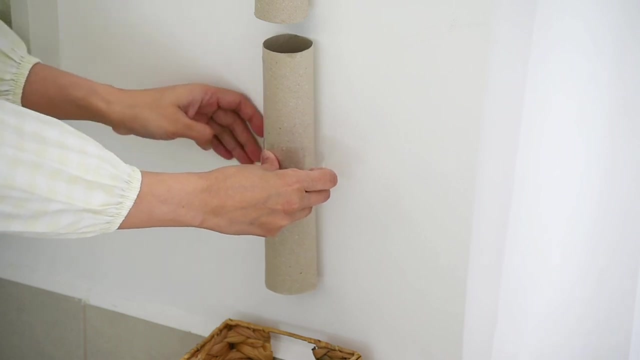 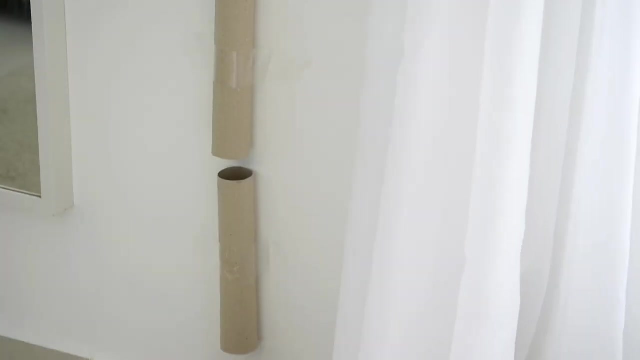 Here is a special video dedicated to all the little ones in your house. In this video, I have included 10 amazing kids activity ideas that can keep them happy and busy for some time. First one is a tissue paper roll activity. For this, you just have to stick the tissue paper roll on the wall. I stuck two of them, but 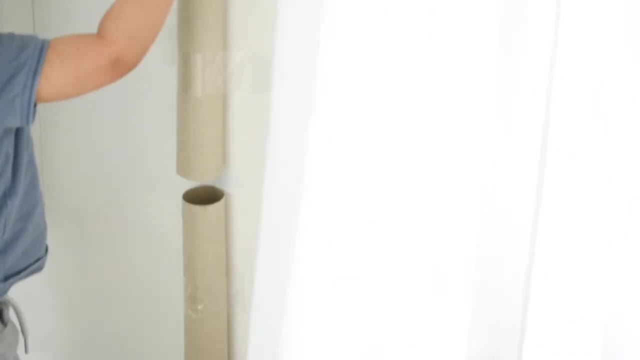 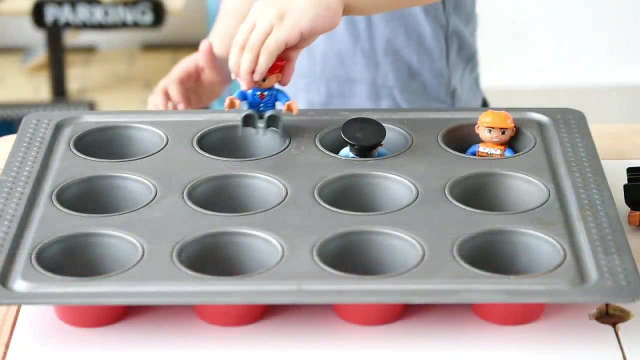 you can just do it with one and place a basket underneath, Give them balls or lego pieces and ask them to throw it through the tube, and they will be very excited to see it falling into the basket. Next one is save the trapped animal or people activity. For this you'll need a cupcake. 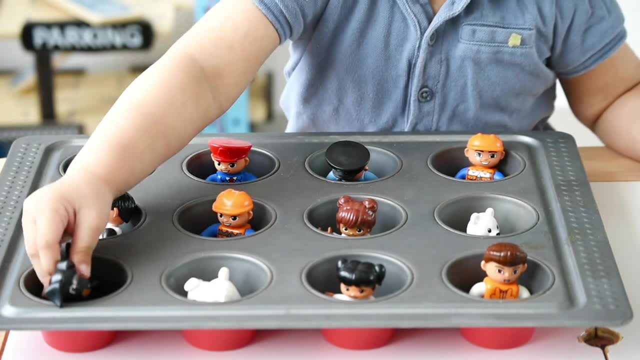 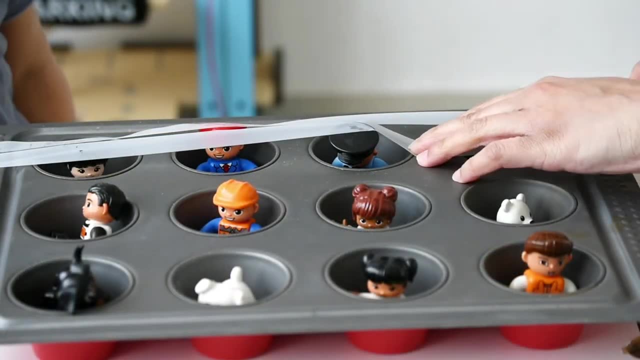 tray and small animal toys. You can also use a plastic bag or a plastic bag. You can also use small toys or human toys like this. I'm using the lego minifigures here. Then I pretended that I'm trapping all these minifigures inside the tray with this tape. 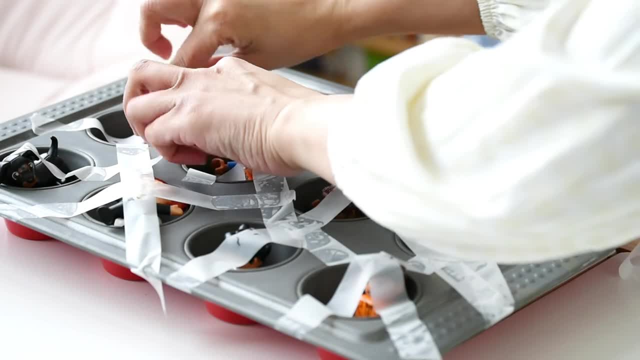 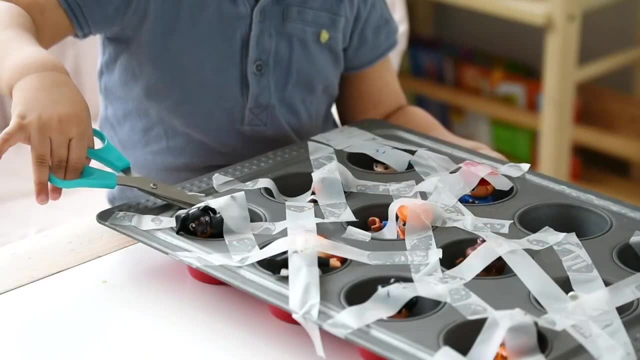 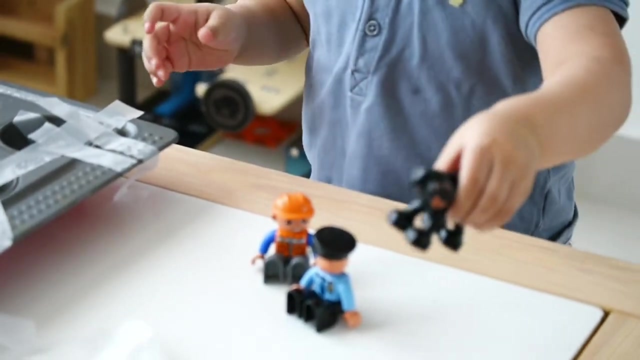 Then I asked Omar to save these people by cutting the tape. If your kid is not familiar with using the usual scissors, please don't give it to them. It would be better that you give them the safety scissors, or you don't even need the scissors, You can just ask them to. 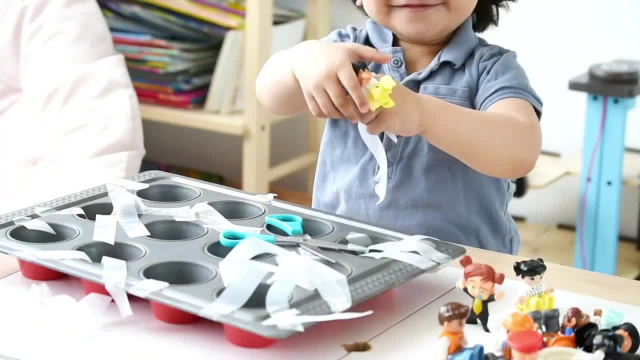 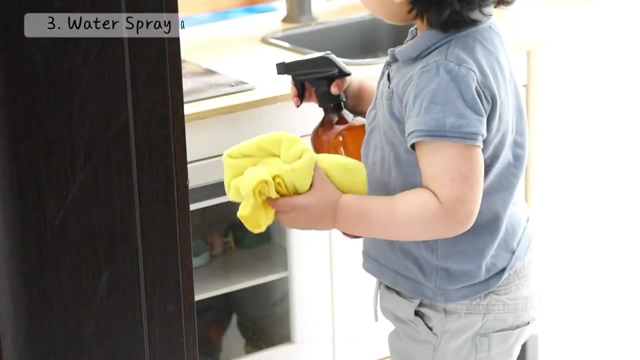 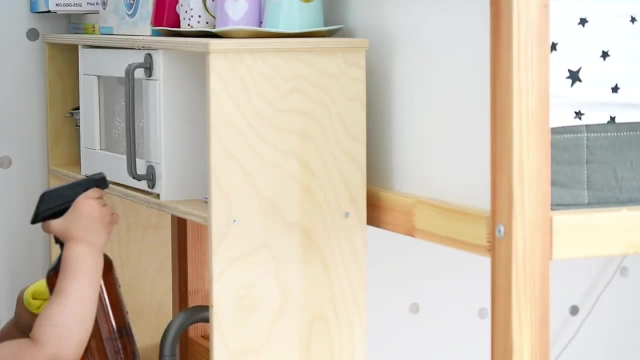 take off the sticker and save the animals or the humans. This water spraying and cleaning activity is a lifesaver. This keeps most kids busy for a long time. I just filled up the bin with water and I'm going to put it in the bin. I'm going to put 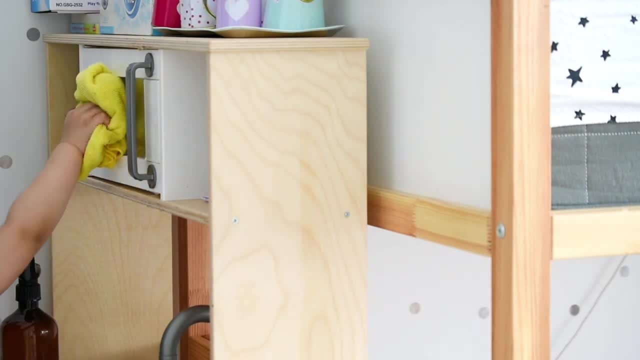 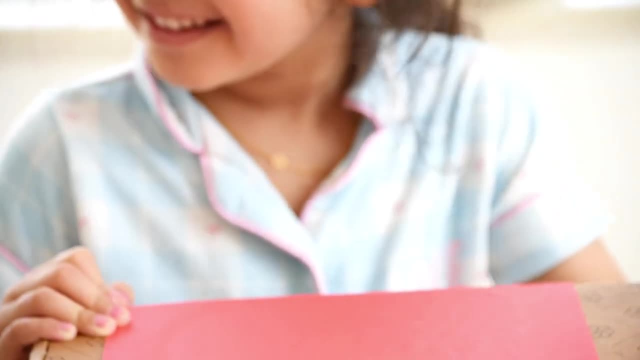 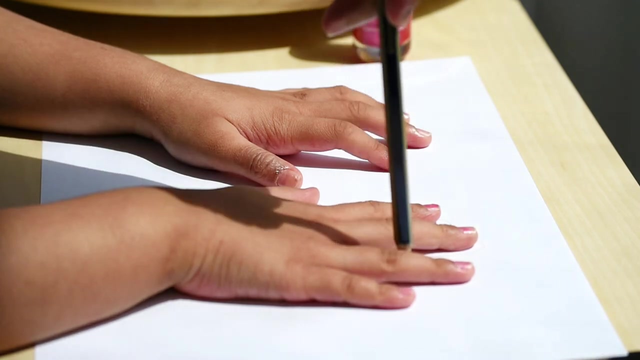 a spray bottle with normal water and give them a cloth and they can just spray it anywhere and wipe it. Hello everyone, this is Aisha doing activities. So Aisha entered the scene and she wanted to give an introduction, So this activity is Aisha's favorite. What I do is I just draw an. 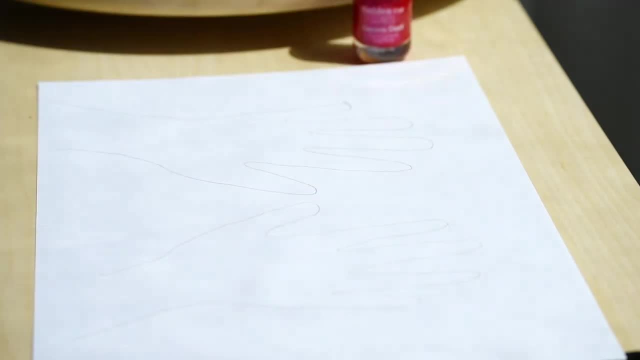 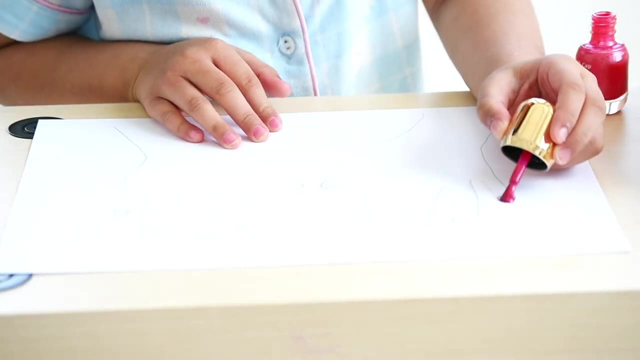 outline of her hand and draw nails on top of it. Then she just paints the nails with her nail polish. I mostly take a big roll of paper and draw lots of hands on top of it and give her different color nail polish And then she plays. 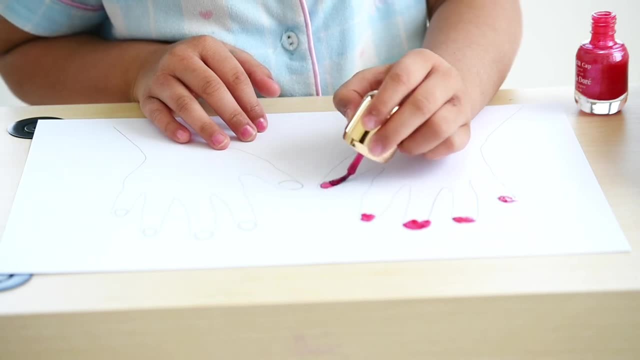 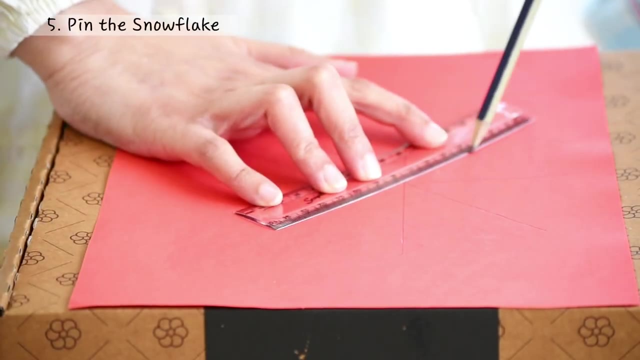 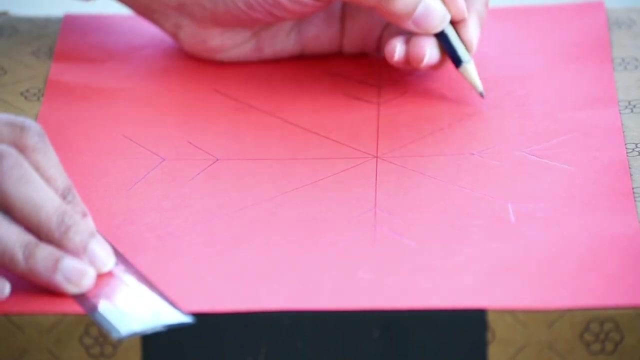 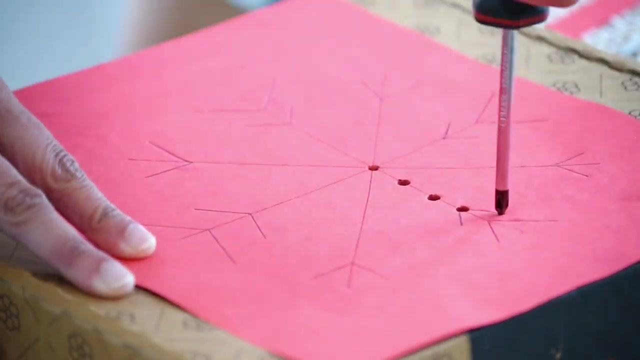 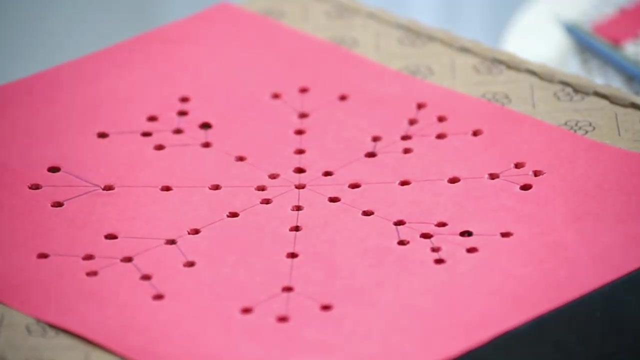 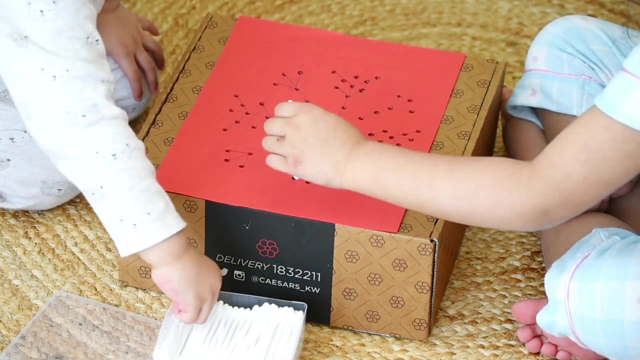 with it. Next one is spin the snowflake activity. For this you need a cardboard box. I stuck a paper on top of it and drew a snowflake pattern. Then I made holes with a screwdriver. I then gave them cotton earbuds and they had to just insert it into the holes. Once you make this, 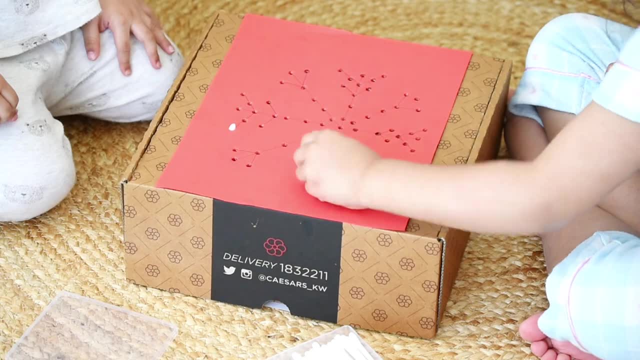 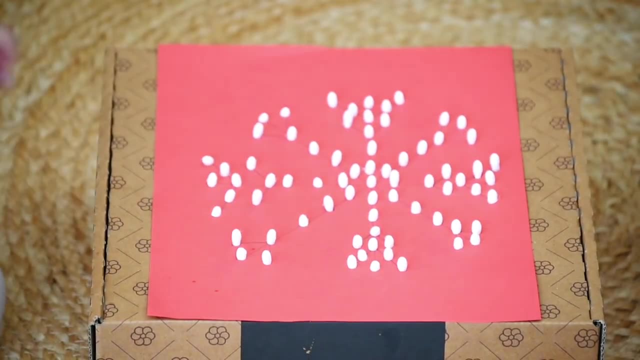 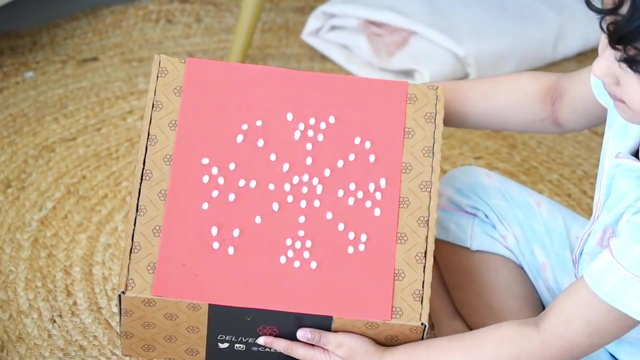 you can save this box and use it later again. You can even use the earbuds again. nothing goes into waste. Instead of snowflake, you can even draw a snowflake pattern on top of it. So this is Aisha's sheep pattern, or anything else Actually. if you don't know how to draw, well, you can even print it. 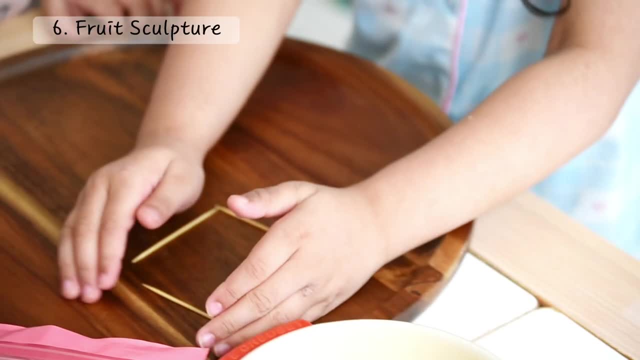 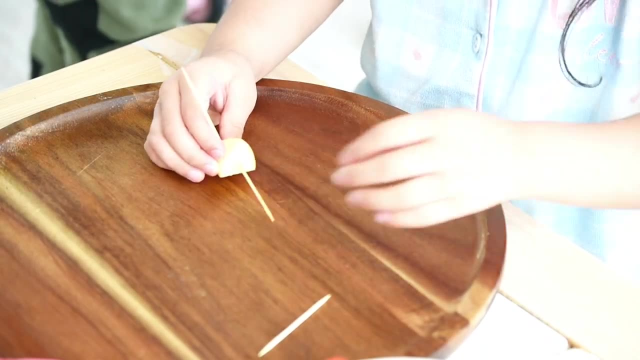 and stick it on the box. By making this fruit sculpture, the children can bring out their creativity by making different patterns with fruits and toothpicks. I have used apples cut in small cubes here, but you can also use grapes or carrots, or even marshmallows. 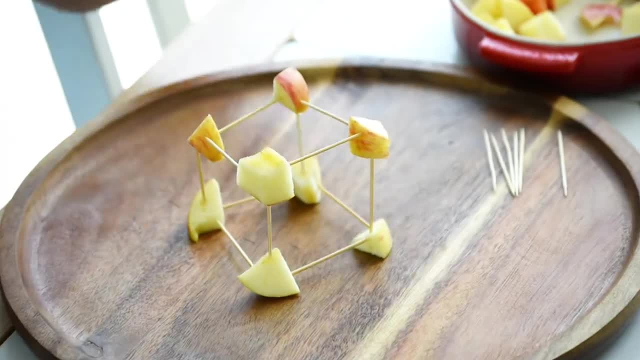 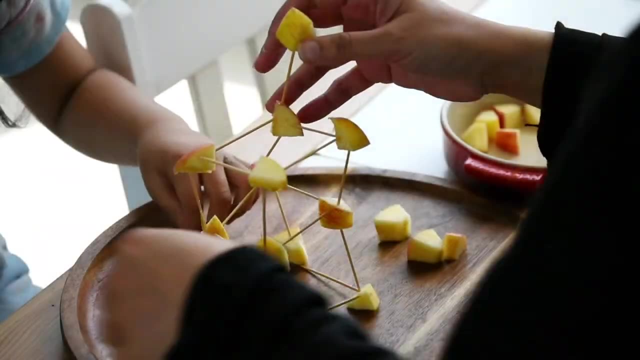 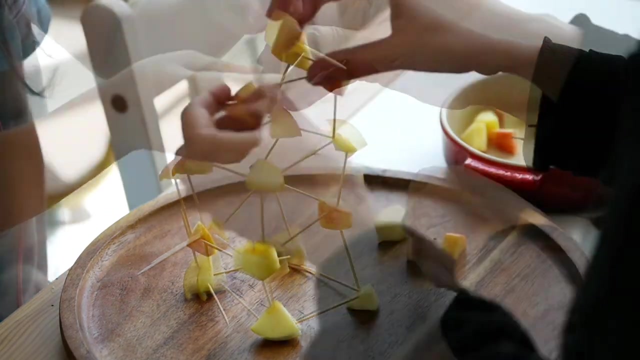 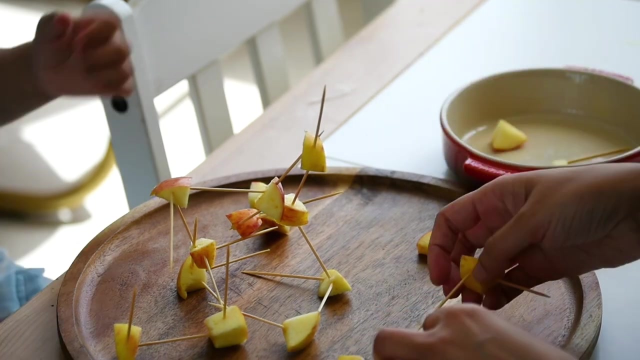 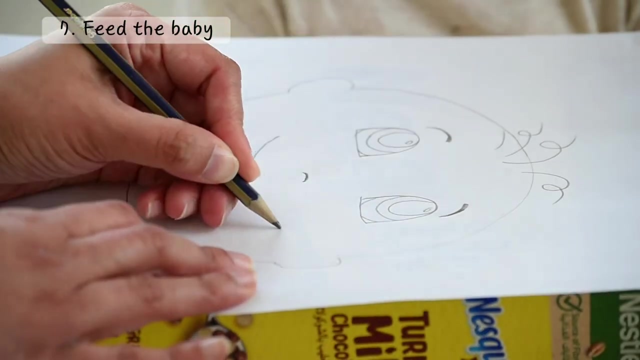 Beautiful sheep that you made. Do you want to make it bigger? Make it bigger. Okay, sorry, we don't need to make it bigger, Mama. Oh, you can just eat it now, Mama. Next one is feed the baby activity. For this, I took a cereal box and stuck a paper on top of it. 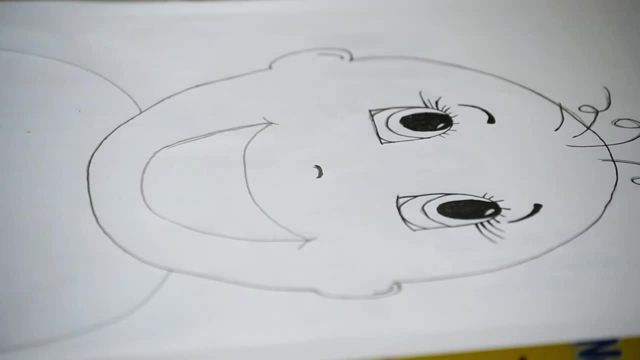 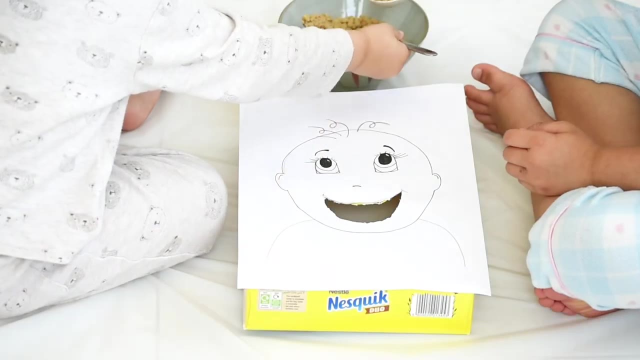 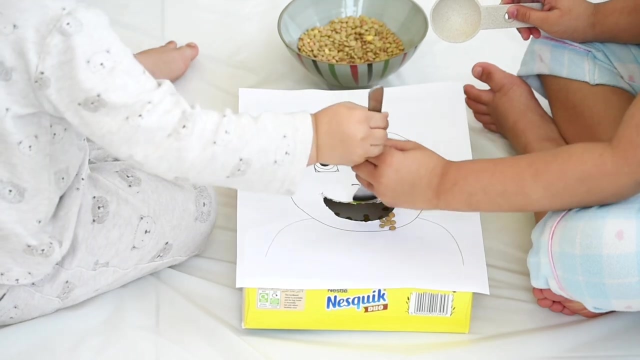 and drew this rather spooky looking baby. I then cut the mouth part of it with this pen knife. The kids were then having a fun time feeding the baby. I gave them lentils. Once the food gets over, you can tip back whatever is there inside the box into the plate again and the children can.